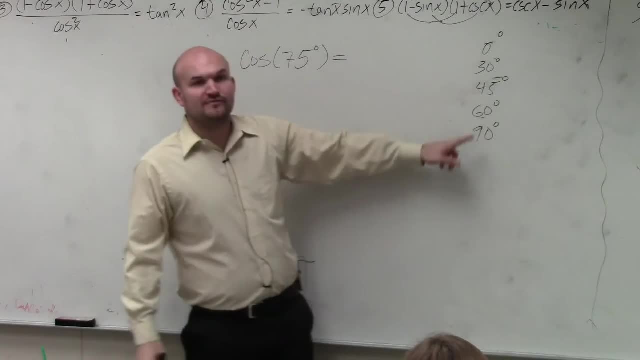 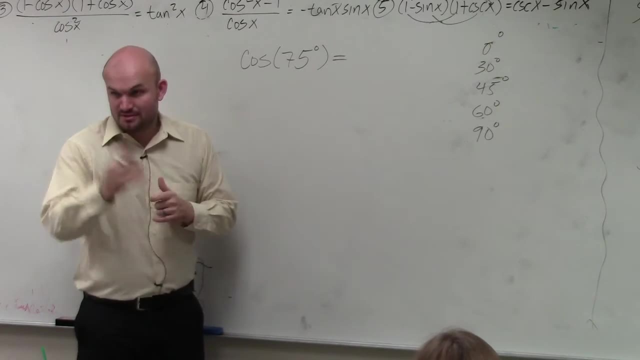 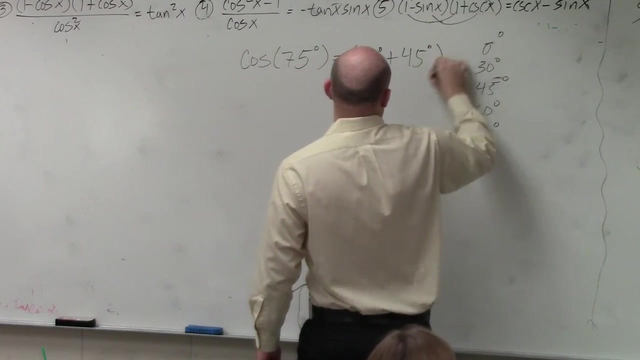 And 90 degrees. That's all the angles in the first quadrant, correct? Can we rewrite 75 degrees as a sum or difference of two of those angles, 30 and 45. So what you're going to do is a lot of times they'll be provided for you. So I'm not really. 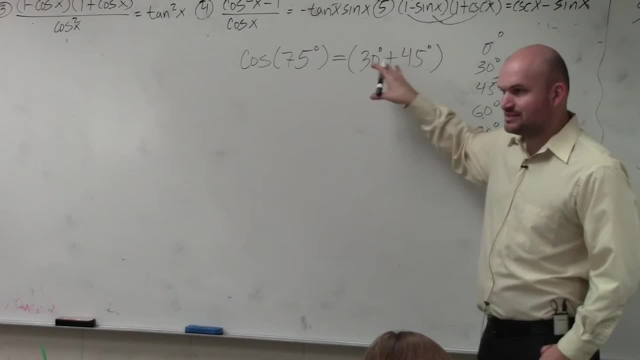 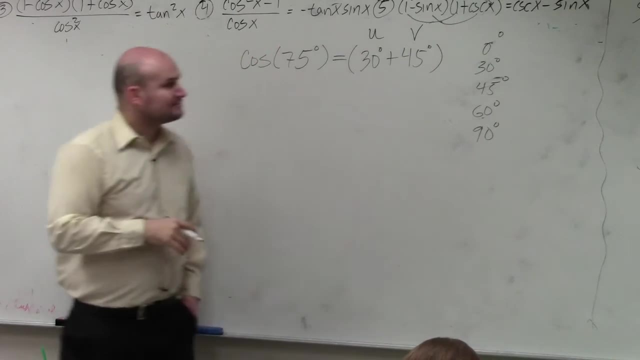 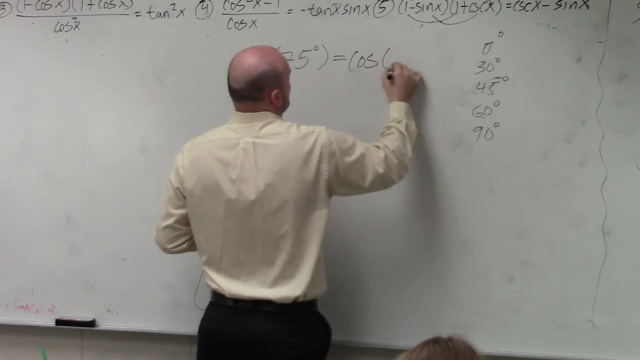 concerned about you guys finding what those two angles are. but does that make sense? That's the same thing. So guess what? Once we do that, we label one U and one V Here. let me actually write this mathematically correct: That's equal to the cosine of 30. 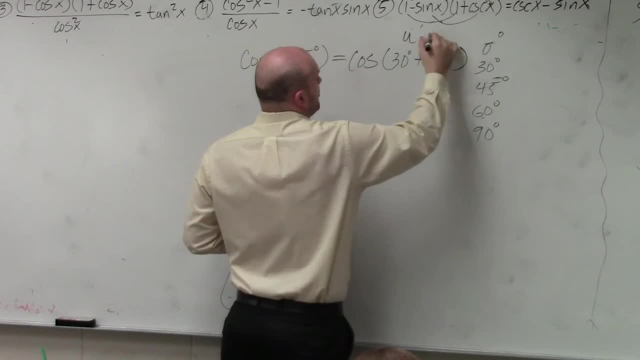 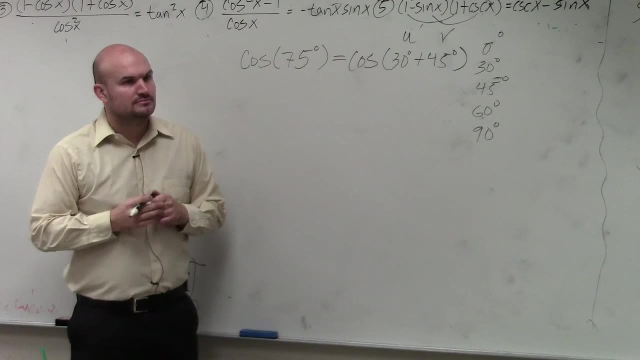 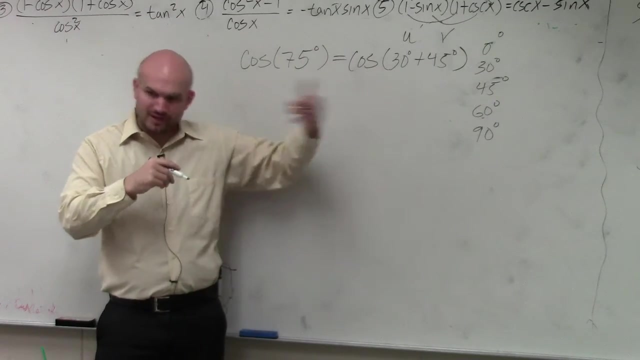 degrees plus 45 degrees. Does it matter which one you look at? Nope, Does not matter. Now, when you're doing subtraction that's a little bit different, because you got to have them, but you got to you. might you want to have U minus V and that's four. So 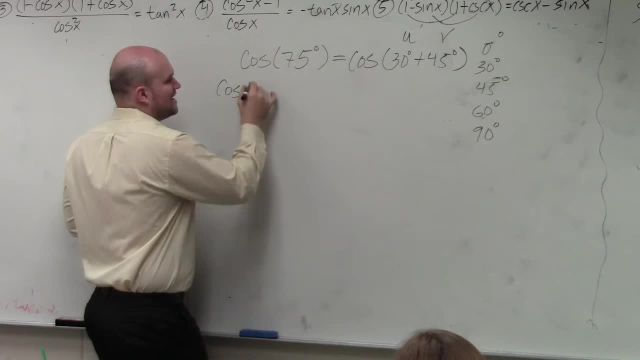 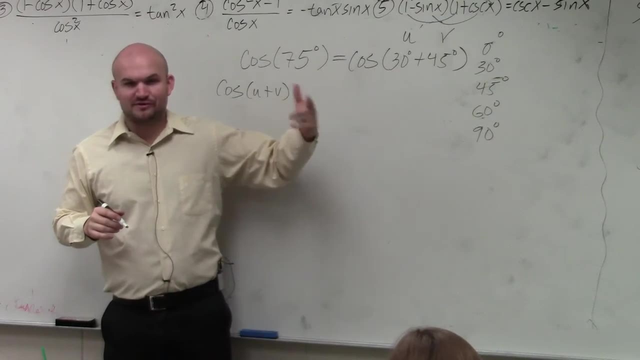 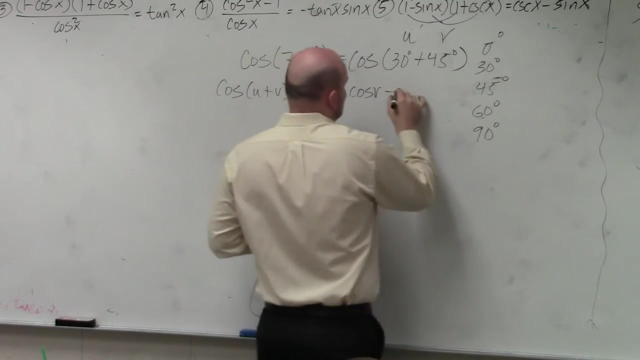 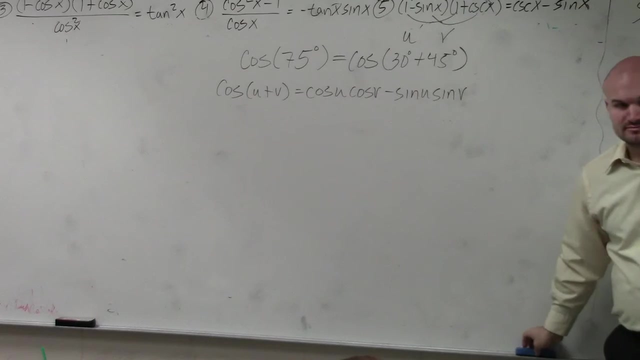 anyways. now we need to go through our formula. So cosine of U plus V- if I remember it correctly, it's cosine of U sine of U minus. no cosine of U. cosine of V minus sine of U sine of V. Okay, Equals cosine of U times cosine of V minus sine of U times sine of V, Right So? 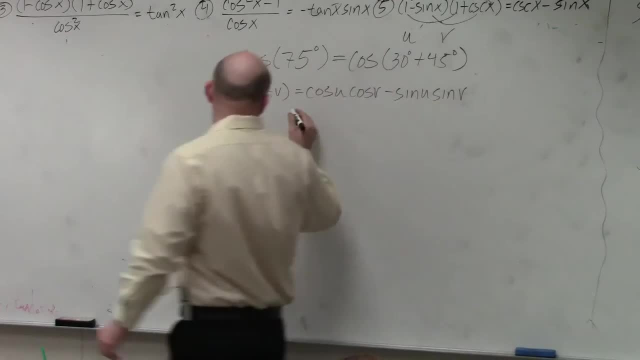 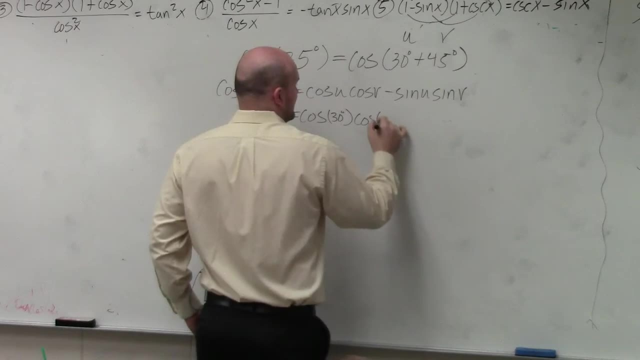 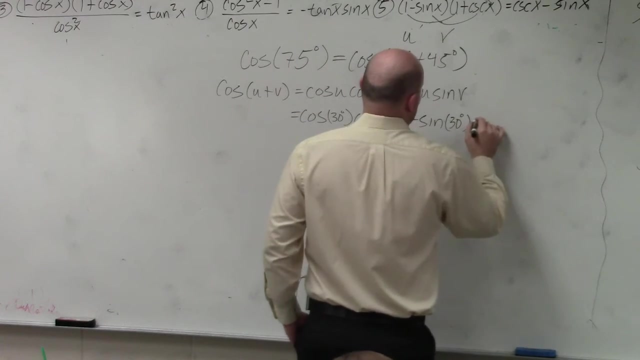 now all you're going to do is just plug in the formula, Use the values that you have. So we have: the cosine of U is 30 degrees times the cosine of V is 45 degrees, minus the sine of U, which is 30 degrees times the sine of V, which is 45 degrees. Now do you guys see how we have? 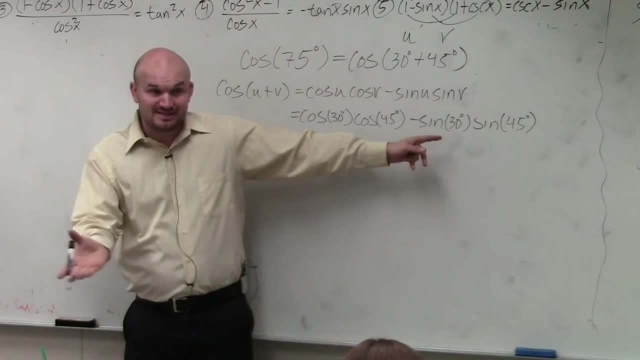 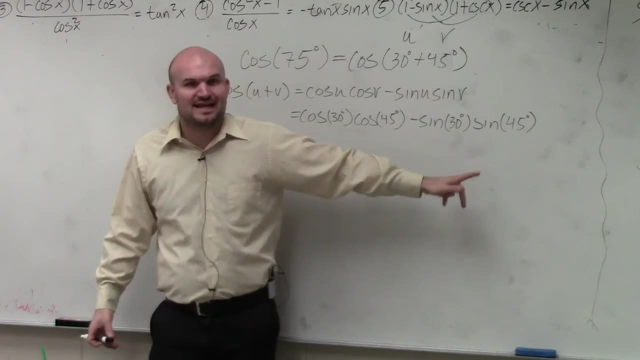 to evaluate one, two, three, four- kind of like four- problems on your guys' test, right? Really, it's the same thing. That's what I'm asking you guys to do, But you guys need to be able to do this without spending 20 minutes sketching the angle. 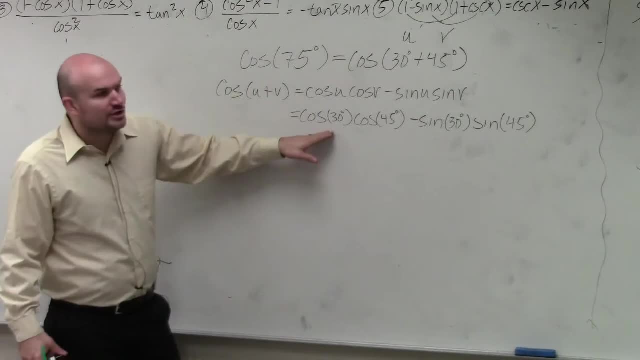 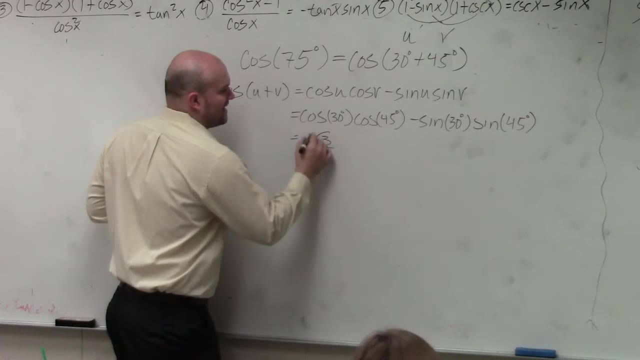 Finding where it is on the unit circle and so forth. You guys should know cosine of 30 degrees. Let's go and get through this. So, therefore, this is going to become the square of three over two, And these are all in the fourth quadrant, So these are obviously easier. 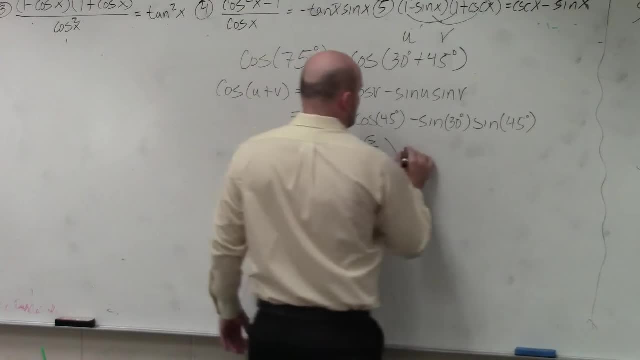 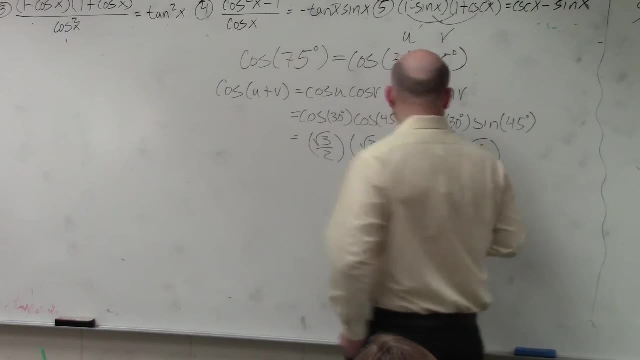 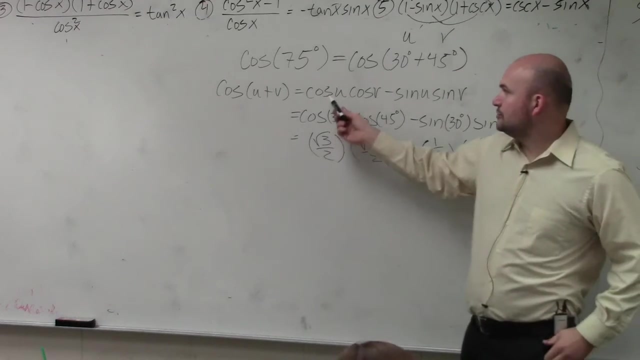 than what was on your quiz. Square root of two over two minus sine is one half times square root of two over two. Does everybody agree with me on this? Okay, Do you understand how I broke up 75 degrees to 30 and 45?? Do you agree with me that formula? 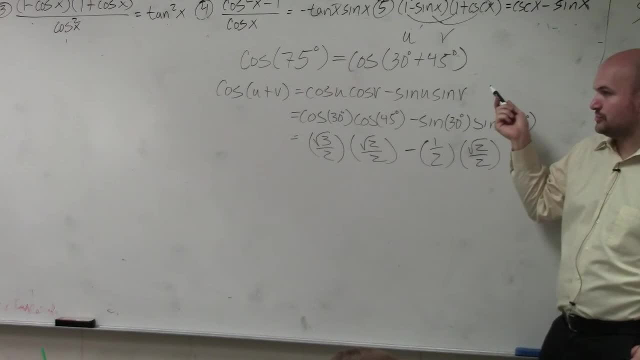 was provided to you. I gave you that formula. That's why I told you to write down Cosine of U plus V. But why does it say cosine of U minus sine of V, sine of V? All right? Well, this is the whole formula I wrote down. so you want to make sure you. 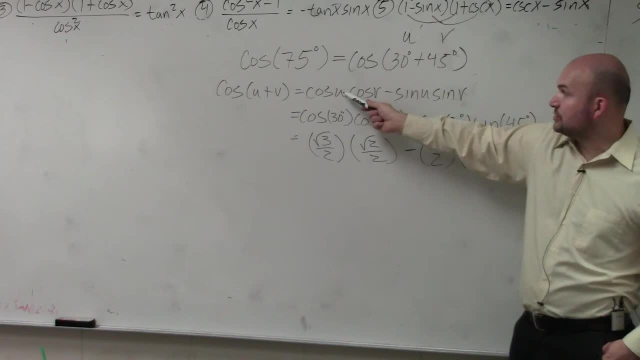 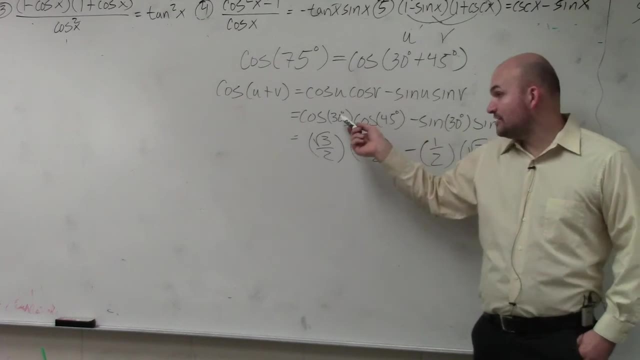 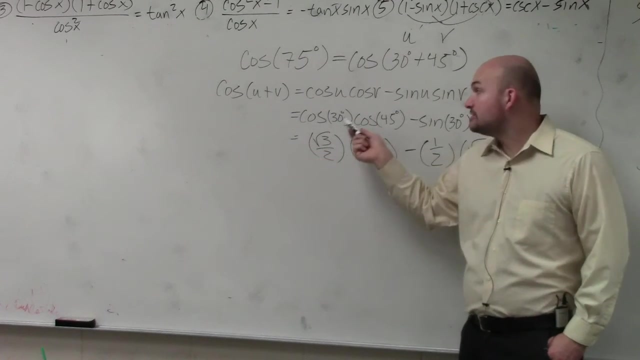 have the whole thing written down. And then all I did was, wherever there was a U, I replaced that with 30 degrees. Now, the cosine of 30 degrees, remember, is the x-coordinate of the coordinate point where the angle 30 degrees crosses the unit circle. So if you look on your unit circle, 30 degrees, 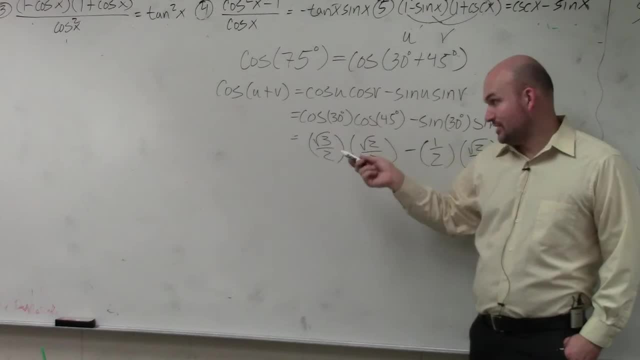 the cosine is the x-coordinate, which is square root of 3 over 2.. If you look on your unit circle, cosine of 30 degrees is square root of 3 over 2.. Cosine of 45 degrees, So forth. 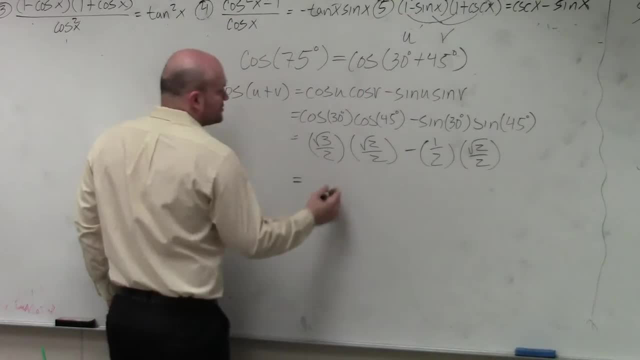 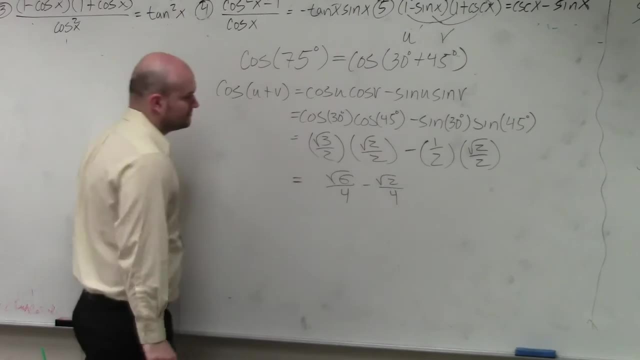 Now we just need to do our math to simplify. So therefore we have square root of 6 over 4, minus the square root of 2.. Thanks, guys, 2 over 4.. That is one answer. That's perfectly fine. 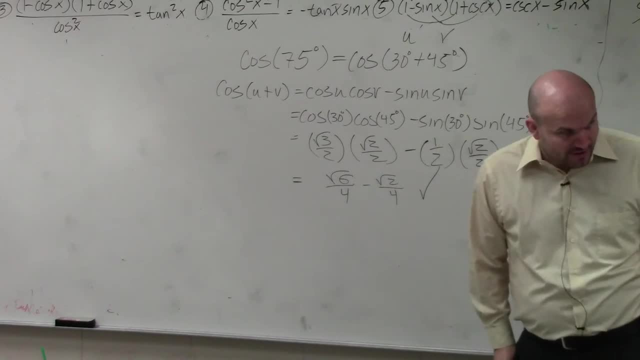 However, they might ask you to simplify this even further. So I'm not sure even how the book writes it out there. Actually, let me look at what the book writes it. No, they leave it like that, But some books or some answers on your end of the year test. 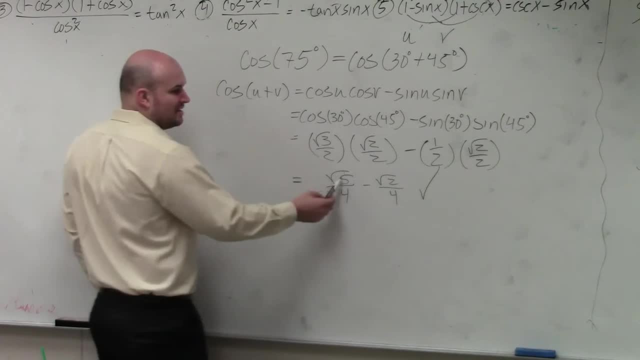 I'm not sure They might also have you factor out common terms. Is there a radical that you can divide evenly to the square root of 6 and square root of 2?? Square root of 2.. So you could factor out the square root of 2 and 4.. 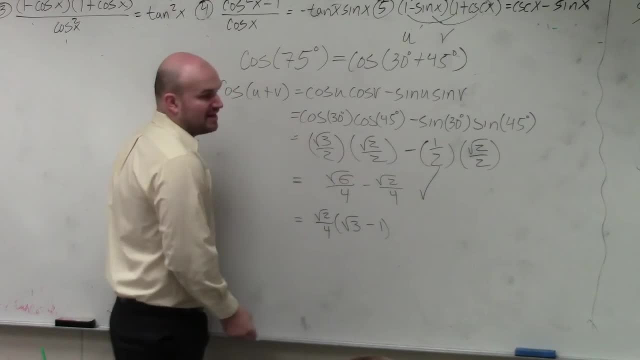 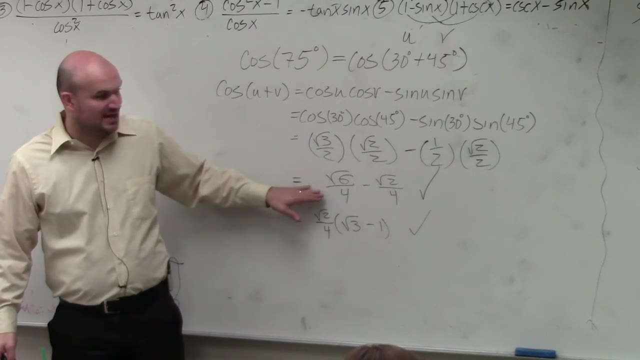 And that would leave you with the square root of 3 minus 1.. Just know that is another simplified way. The book has this as their answer, So I'll be OK with you guys if you want to leave your answer like this. However, just note you might have a test.